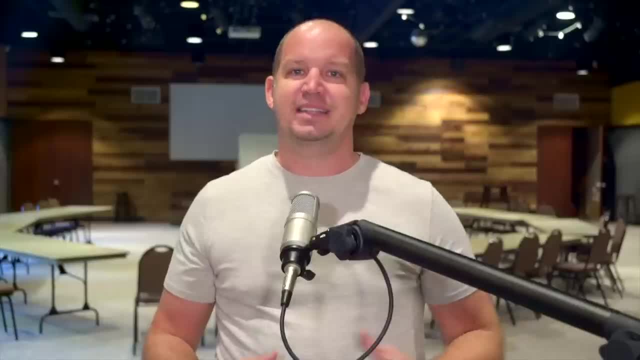 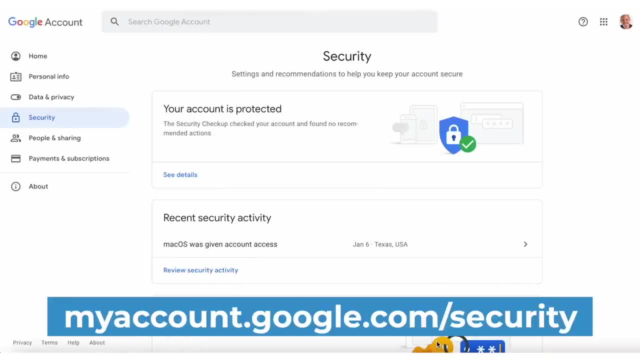 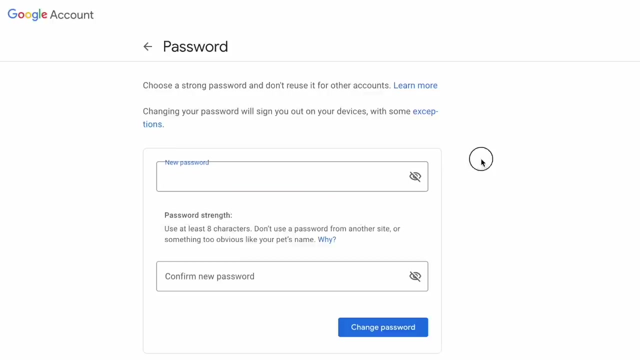 of characters, the longer the better. that is unique, meaning that you only use that password for Gmail and not a single other online login. To change your Gmail password, go to myaccountgooglecom slash security and click on password under signing into Google. Make sure you create a better password that you won't forget and that isn't used. 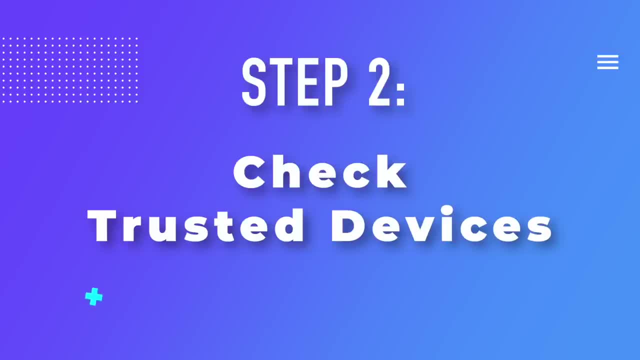 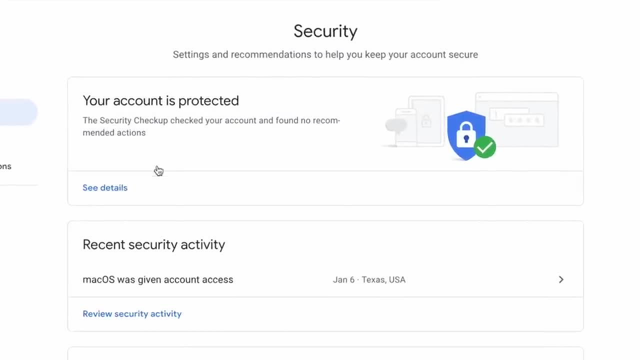 anywhere else. Now that you're in your security settings of your Gmail account, you may have noticed a few warnings under the security checkup box. Even if Google gives you a pat on the back with your message reading your account is protected, I still recommend you jump over. 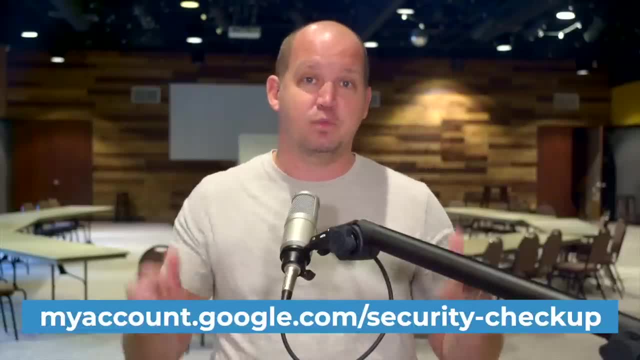 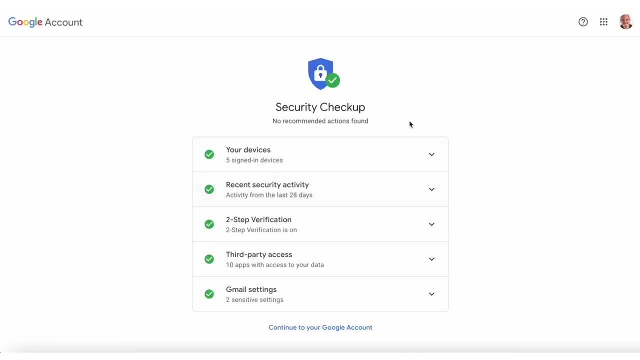 to the security checkup page. I'll have a link in the description or in the description where you can just type in what you see here on the screen. It's really important to know what you can do with this tool that Google provides, both from a monitoring and from a threat avoidance standpoint. For example, I can check all of 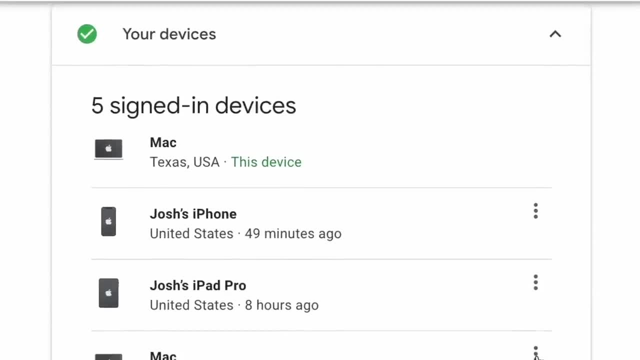 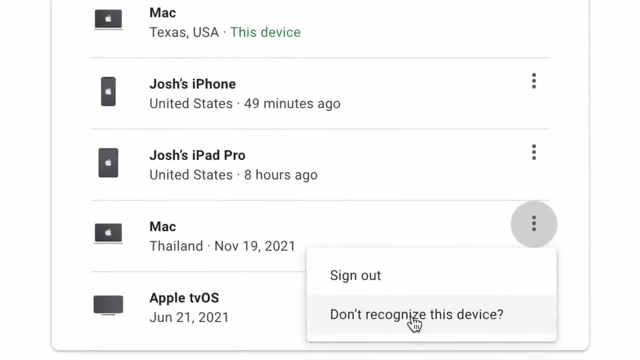 the devices that are listed as trusted, to open my Gmail accounts and to make sure that there aren't any unknown devices that I can tell Google that I don't recognize. Or, better yet, let's say that my phone was stolen or lost. This allows me to quickly. 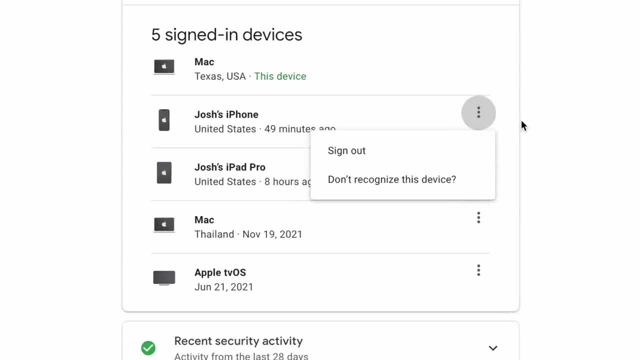 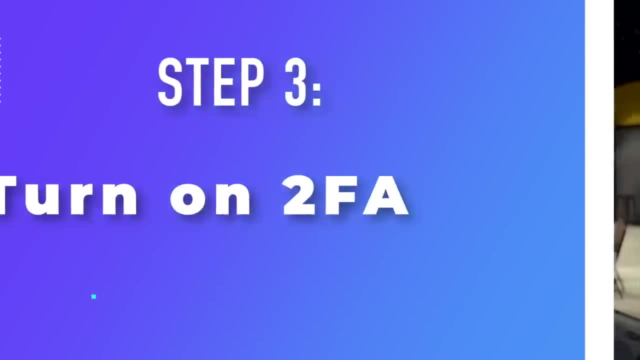 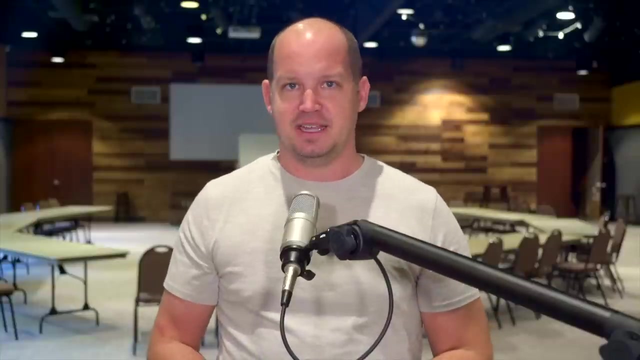 jump in and tell Google to sign that device out so that nobody will have access to my email, even if they're able to get into that device. In my opinion, probably the most important change that you can make to secure your Gmail account is to turn on two-factor authentication. As you can see here, I have multiple security. 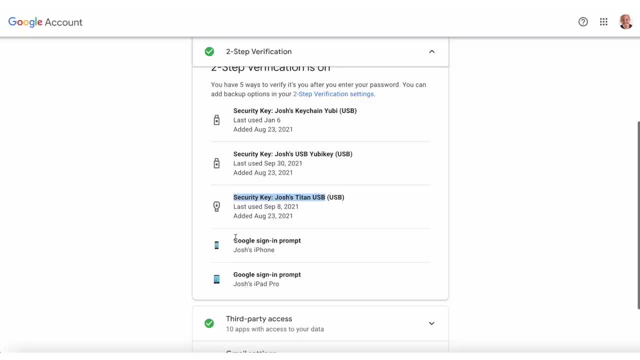 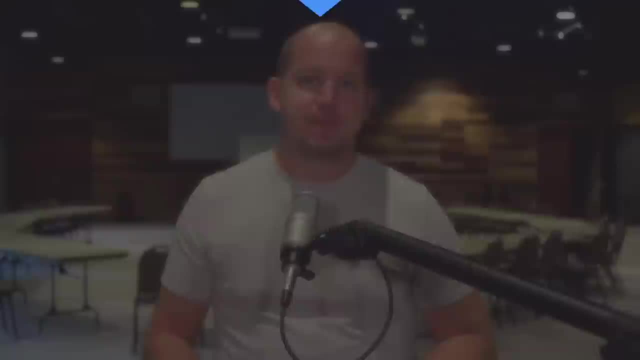 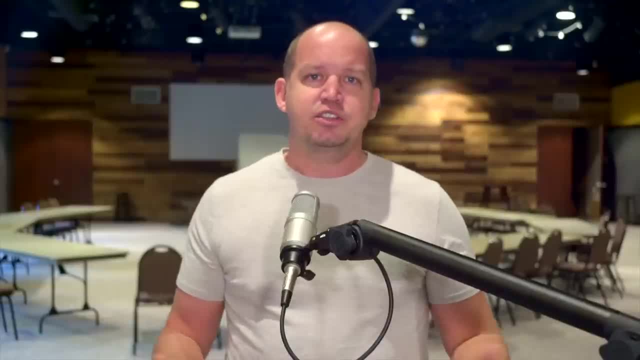 account. If you take away only one thing from this video, I want it to be this: Gmail security does not exist without your Gmail account. If you take away only one thing from this video, I want it to be this: You can use the YubiKey security key to secure not only your Gmail. 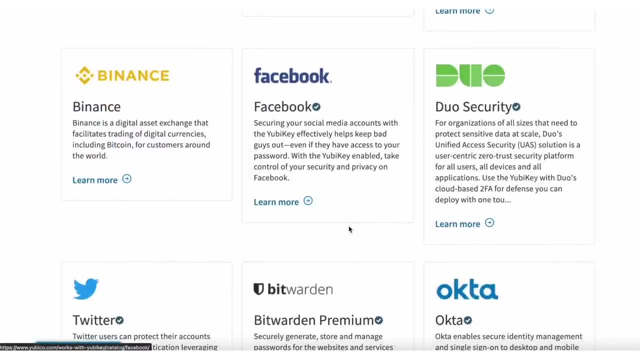 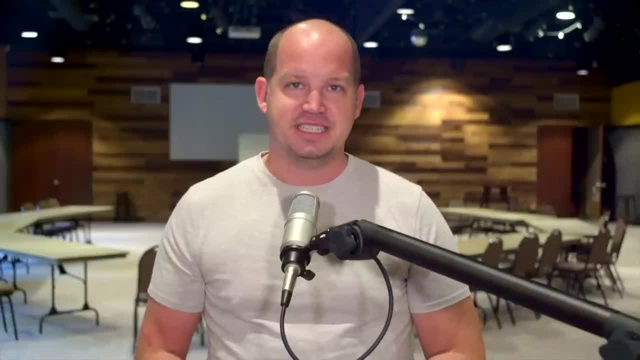 account, but also any other account that supports the FIDO protocol, and there are plenty of them out there. If you don't have your own 2FA key yet, or perhaps you don't have a backup, Yubico is offering a special discount on their affordable security key series that. 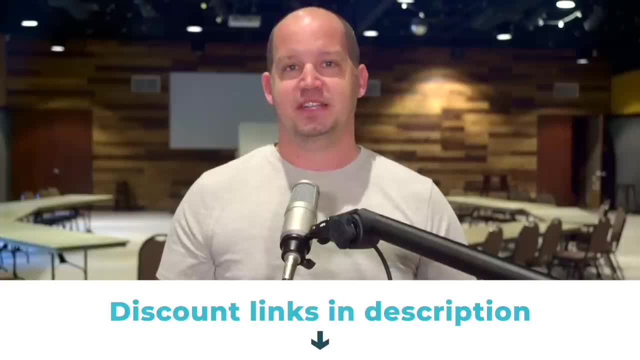 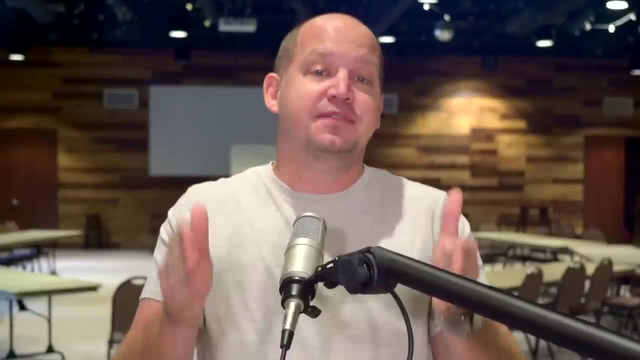 you can buy a couple of your own. You'll find links in the description of this video. Personally, I bought four: a primary and a backup for myself as well as for my wife. I promise you this is an investment in your security that you can't afford neither. 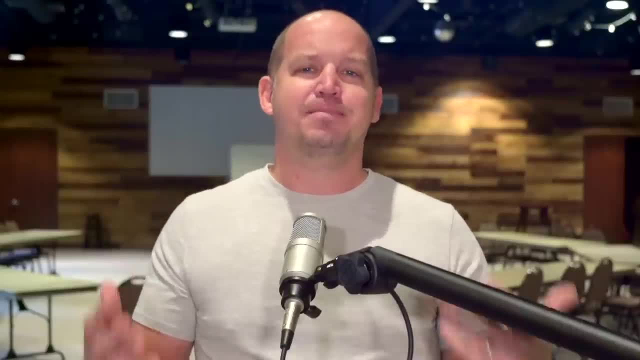 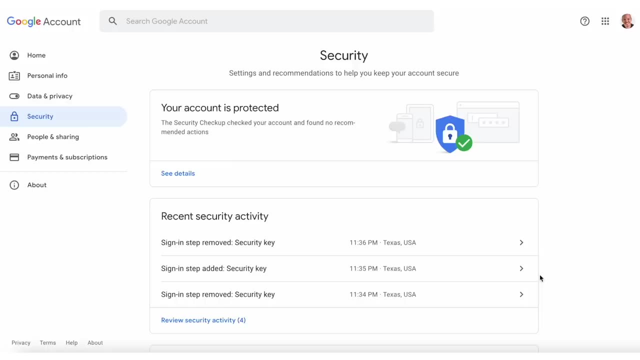 not to make. I know that's a double negative And basically what I'm trying to say is that you need to do this. The process of setting up a 2FA key on your Gmail account is pretty straightforward. Log into your Gmail account, go to myaccountgooglecom slash security. You scroll down. 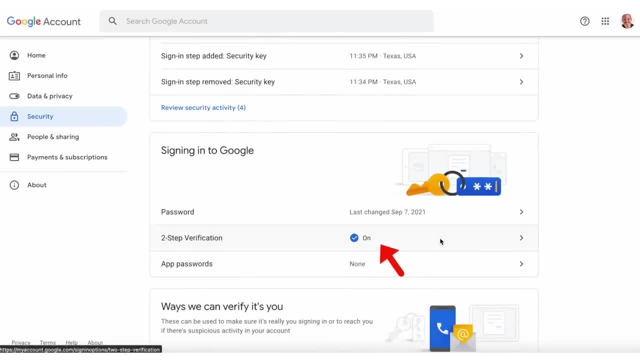 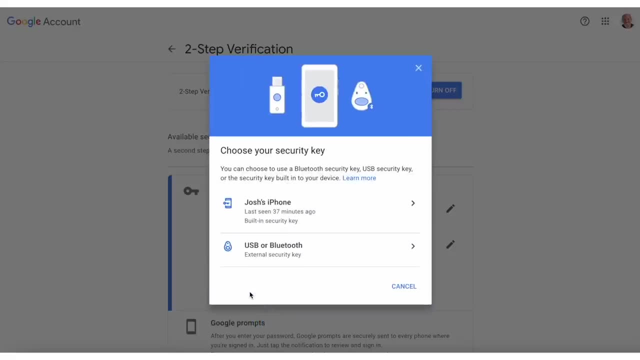 and find two-step verification. You need to turn that on if you haven't already. They call it two-step instead of two-factor. Anyway, you want to add that security key. Of course, you'll already need to have purchased your key, but once you have your YubiKey device in hand, you'll click on. 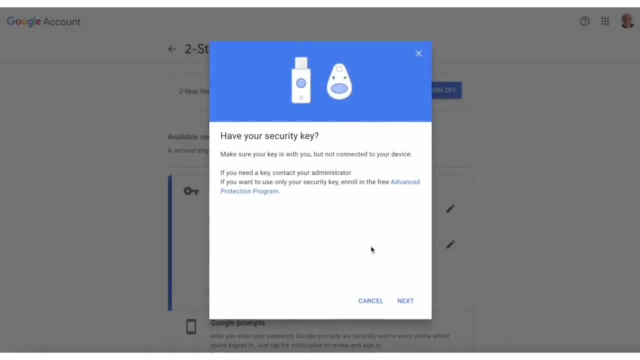 USB and then register the key by plugging it into your computer or device. Name it whatever you want, and then you're done. You can remove these keys from your account at any time, which is useful if you somehow lose that key or it gets stolen, or something like that. Now, anytime that you log, 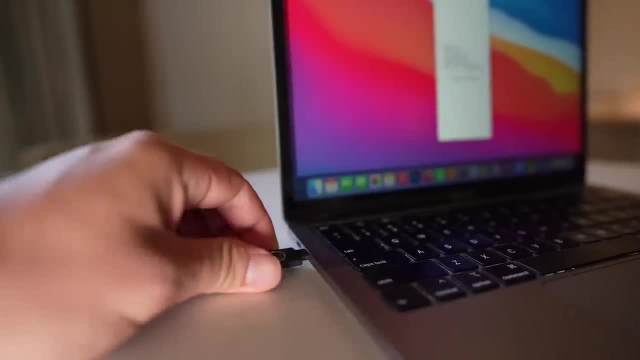 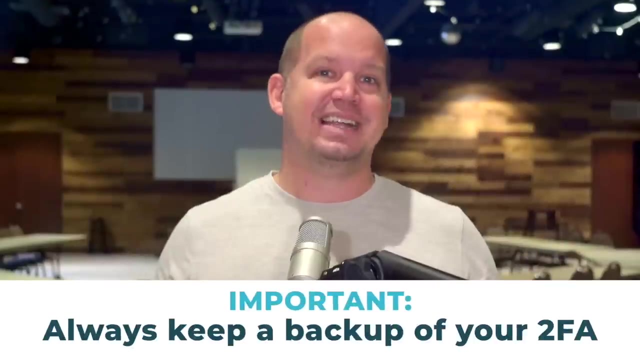 into your email on a new device. you'll need to plug in this key to verify that it is in fact your account. But that's exactly what you want to do. Important side note here: whenever you use any kind of 2FA, you need to make sure you have a backup plan. 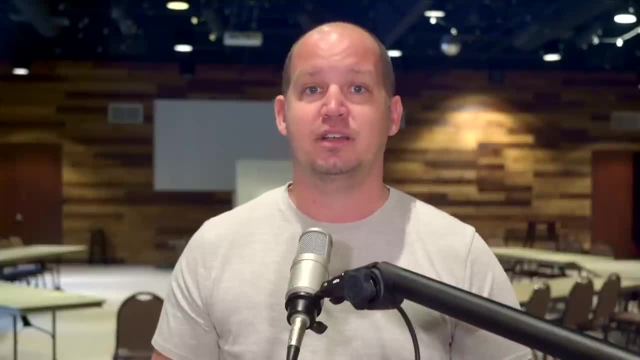 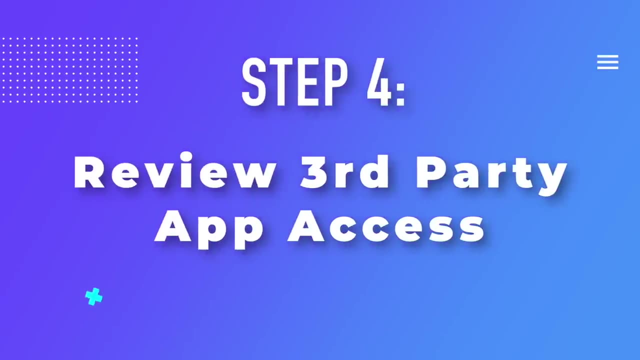 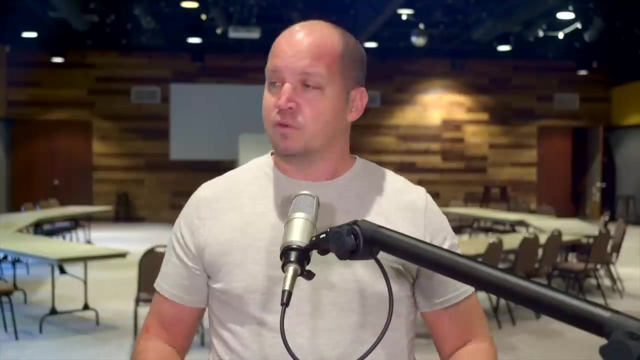 This could be a second key backup codes that you store securely, or something else. The last thing you want, though, is to lock yourself out of your Gmail account. An important step in security checkup after 2FA is to review third-party access Over the years. we all allow certain apps or 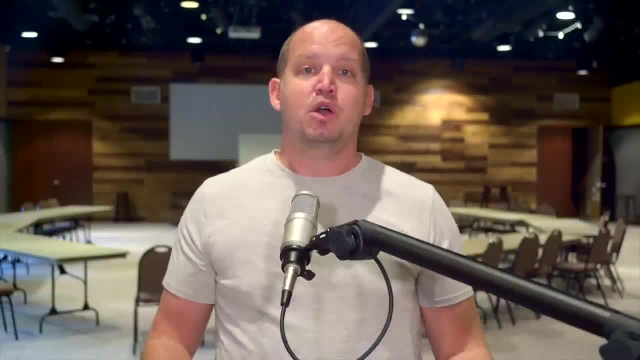 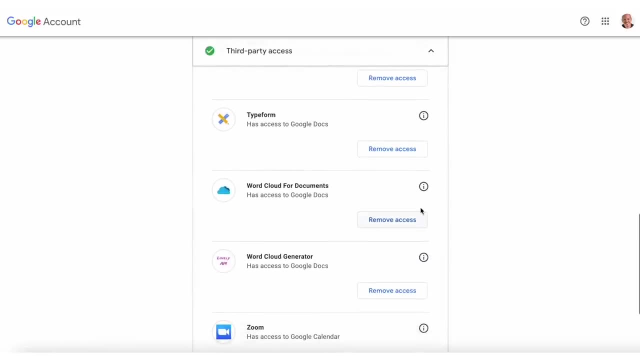 websites to have access to our account and we often forget to remove them when we're done using that particular service. So if you have a security checkup, you need to make sure you have a backup plan. For example, you can see here that at some point I allowed Word Cloud for documents to have. 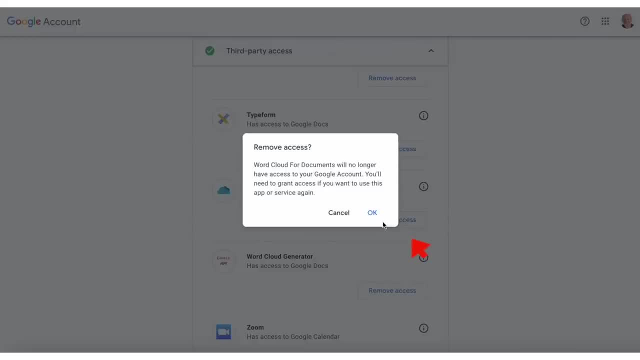 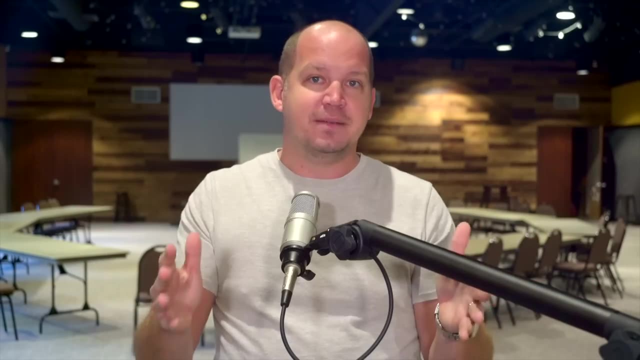 access to my account. Since I don't use that service anymore, I'll go ahead and remove access for them. You should do the same to any apps or sites that you don't recognize, And don't worry if you make a mistake. they can always request new access and you can grant it to them. So